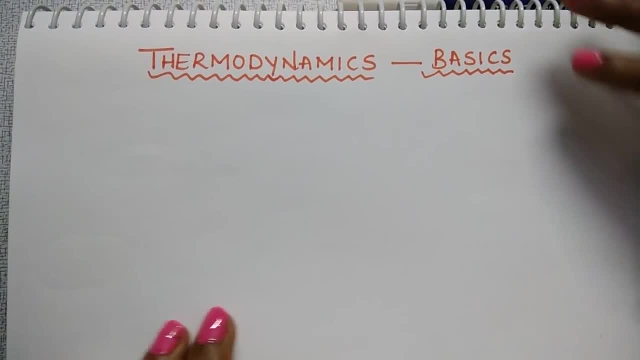 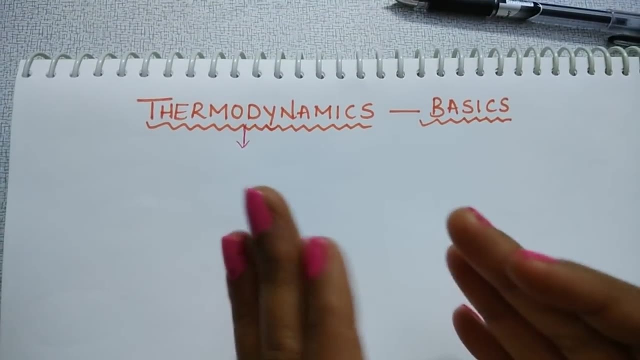 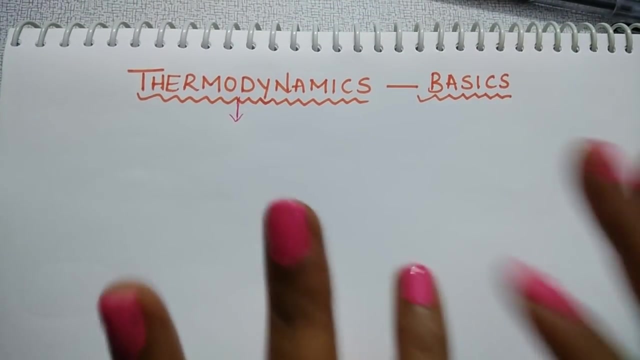 these are very important to understand this chapter better. Let us see first. about what is this thermodynamics? Actually, thermodynamics mainly deals with energy and their interconversions, different forms of energies and their interconversions. Here we study energy in various forms and 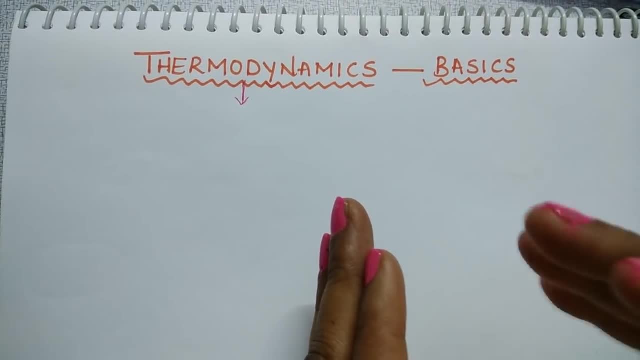 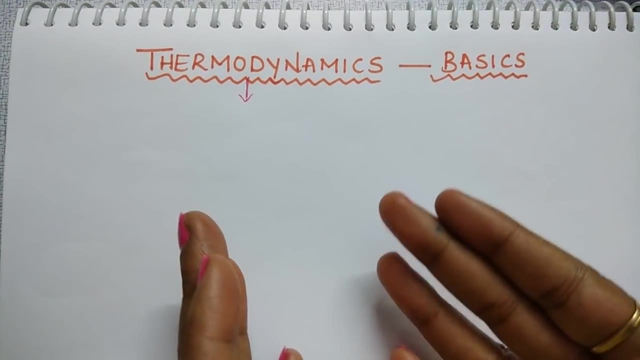 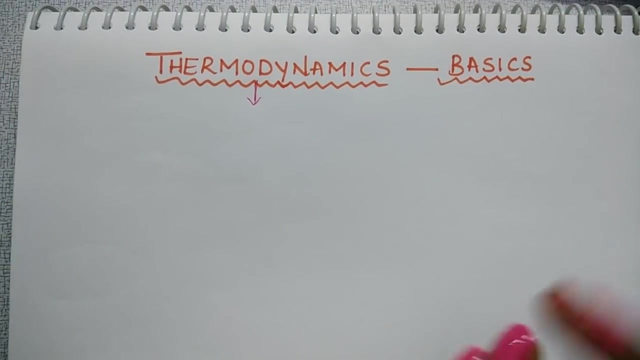 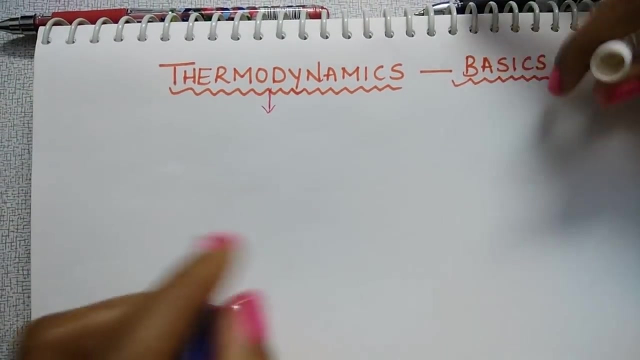 next continuation of this chapter is thermochemistry. There we study energy related to various reactions. Here we study energy in different forms and their interconversions. In thermochemistry we study energy Related to different reactions. Alright, first term which we use in thermodynamics is system. 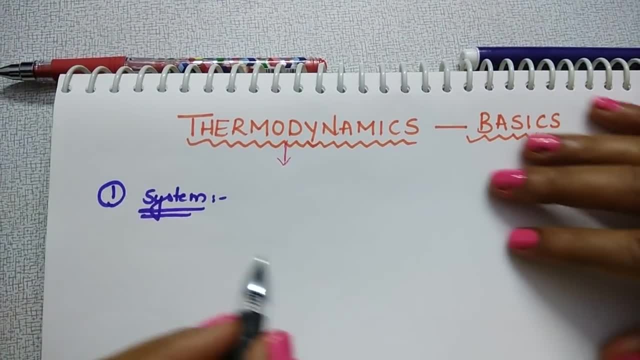 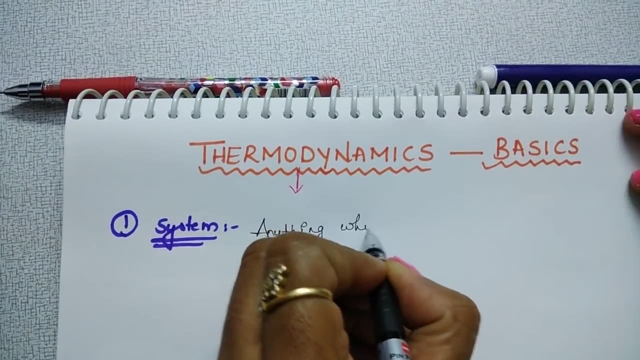